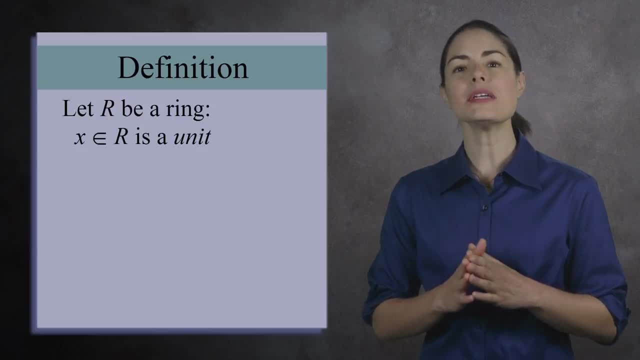 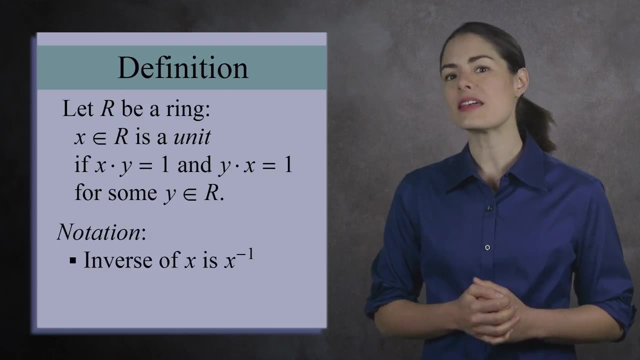 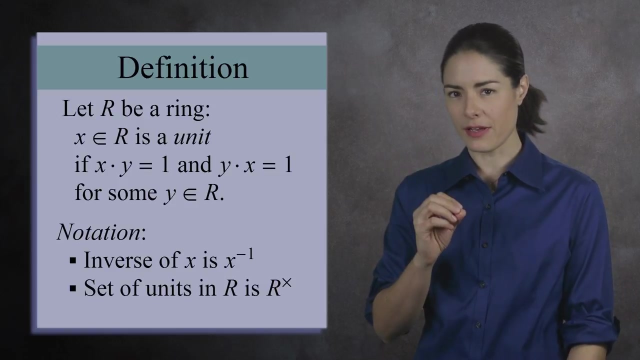 Let R be a ring. An element x is called a unit if there is an element y where x times y equals 1, and y times x equals 1. This is the notation for the inverse of x. The set of all units for the ring R is written with a little multiplication symbol up above. Let's first see a few examples before we talk about the units abstractly. 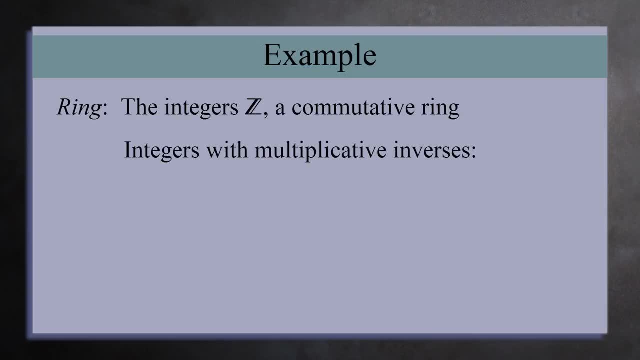 The integers z are a commutative ring. The only numbers with a multiplicative inverse are 1 and negative 1. 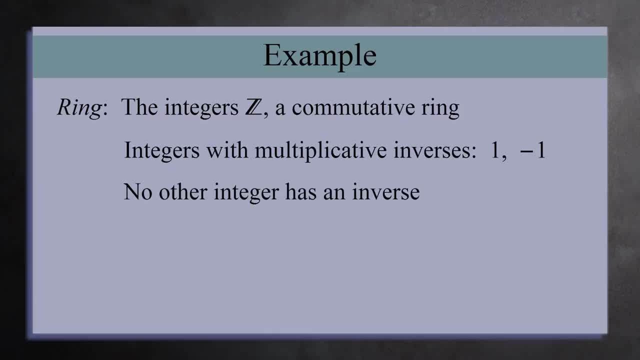 For every other non-zero integer, the inverse would be a fraction, not an integer. For example, the inverse of 3 is one-third, which is not an integer. 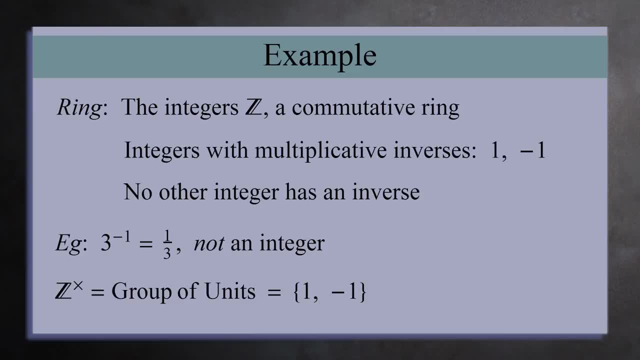 So the units for this ring is a group with only two elements, 1 and negative 1. Here is a group multiplication table for these units. 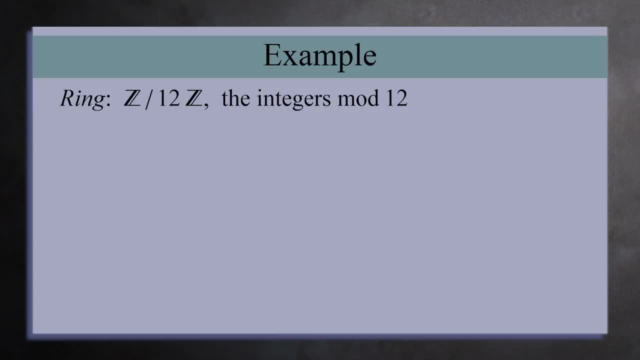 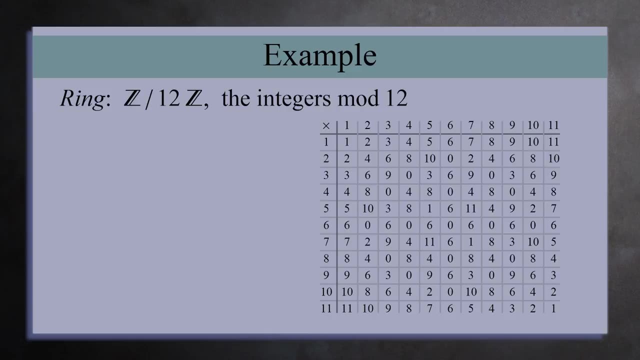 Next, let's look at the integers mod 12. To find the units, let's look at the multiplication table for the non-zero elements 1 through 11. We can find the units by looking for rows or columns at the end of the table. 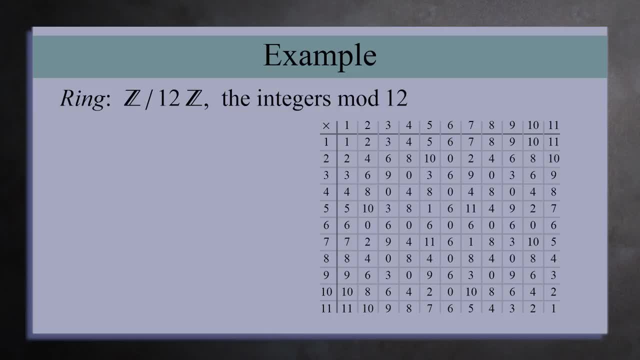 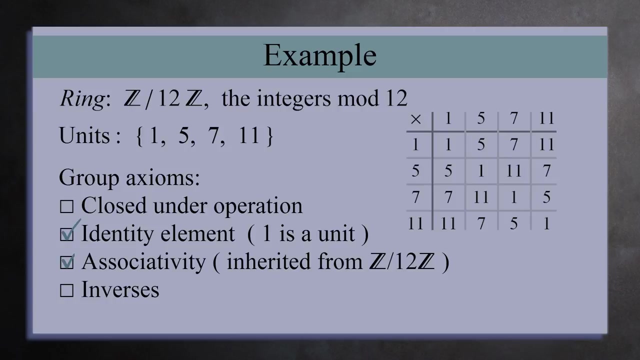 Here are the units that contain the multiplicative identity 1. The only rows and columns that contain a 1 are 1, 5, 7, and 11. These are the four units for the ring of integers mod 12. You can check that this is a group by looking at the group multiplication table for these four units. This table only contains 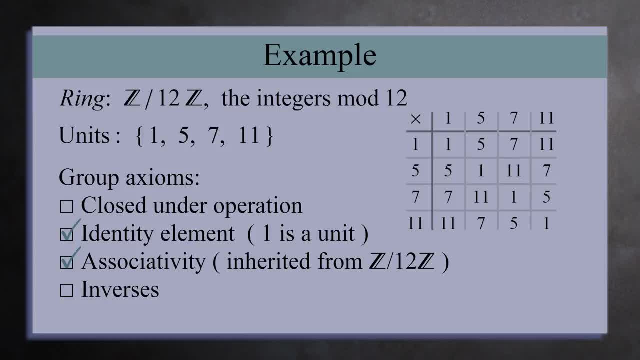 the numbers 1, 5, 7, and 11, so it's closed under multiplication. There's a 1 in every row and column, so each element has an inverse. So the units for the integers mod 12 form a group of order 4. 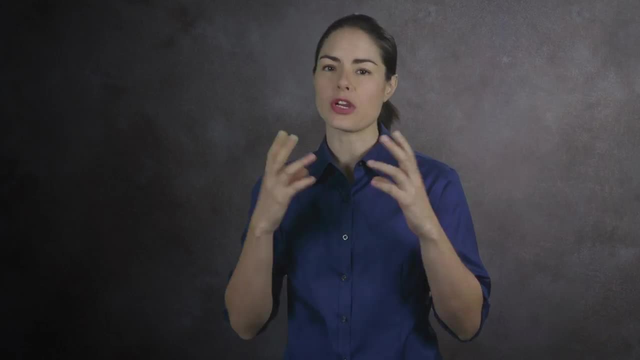 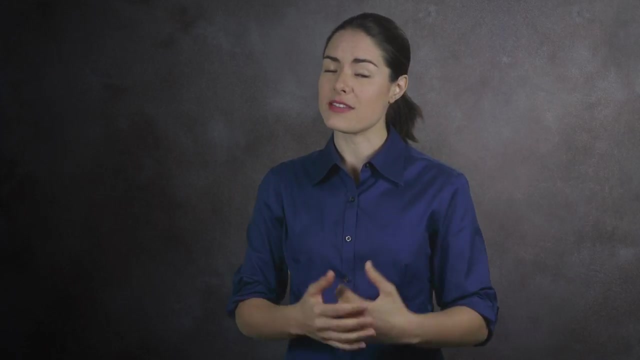 Now that we've seen a couple of examples, let's talk about the units more generally. In the previous examples, we saw that the units form a group under multiplication. Let's now see why this is always true. 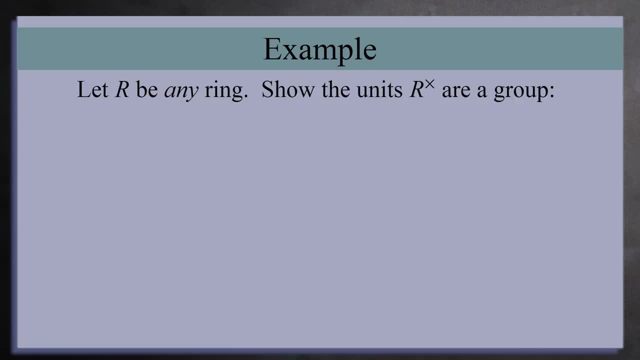 Let R be any ring. Let's look at the set of units and show that it's a group. To do this, we need to check that all the group axioms hold. First, the set of units does contain the identity element 1. So the sum of all the groups can be seen as a group. Then, let's since 1 is its own inverse under multiplication. So this set has an identity. We inherit associativity from the ring R, so we can check that off. Next, by definition, every element x in this set has an inverse y, so we can mark off the inverse axiom. This leaves closure. 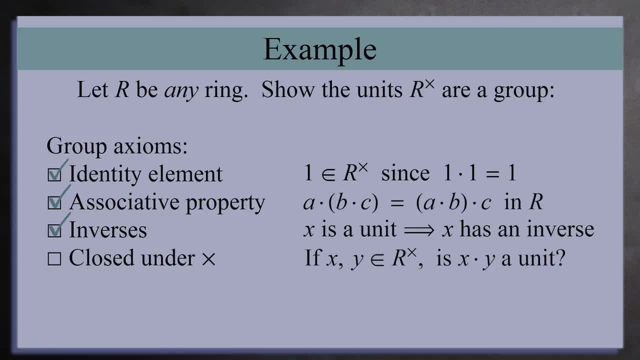 In other words, if x and y are elements in this set, is their product also in the set? That is, if x has an inverse and y has an inverse, does x times y also have an inverse? Indeed it does. The inverse of x times y is y inverse times x inverse. Since x times y has an inverse, it must also be in the set of units, so we have closure. 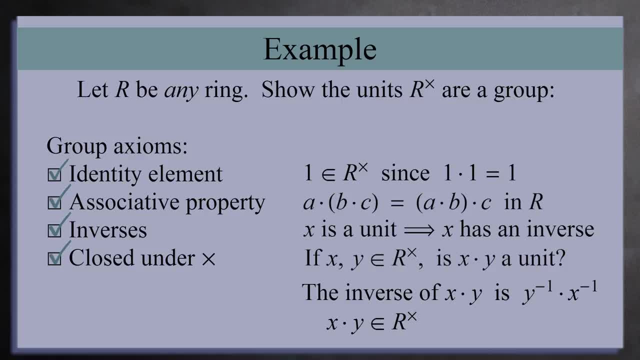 This shows that units do indeed form a group under multiplication. 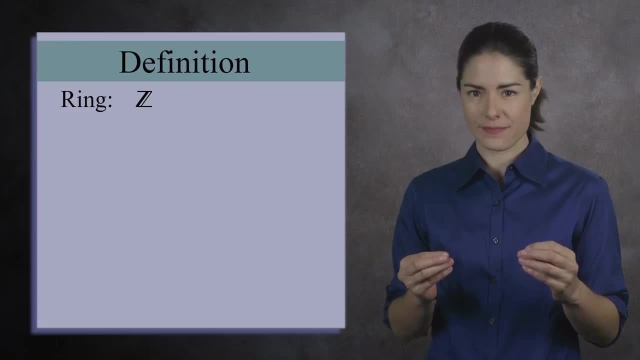 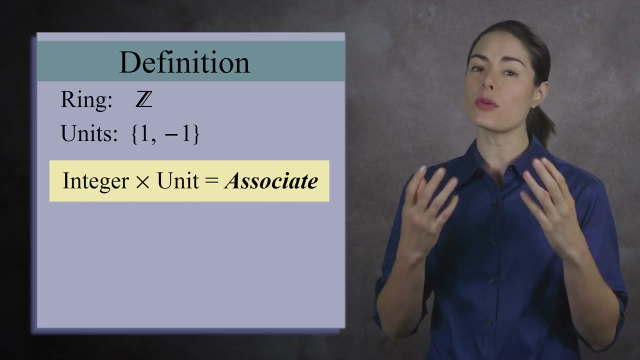 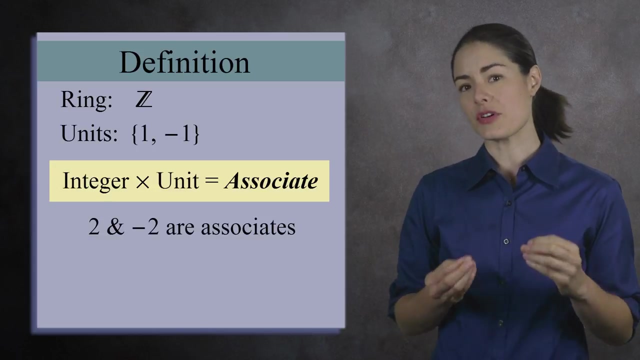 Let's return to the example of the integer z. This ring has two units, 1 and negative 1. If you multiply any integer by a unit, you get what's called an associate. For example, if you multiply the integer 2 by the integer 1, you get 2 and negative 2. These integers are associates. Similarly, 3 and negative 3 are associates, as are 4 and negative 4, and so on. 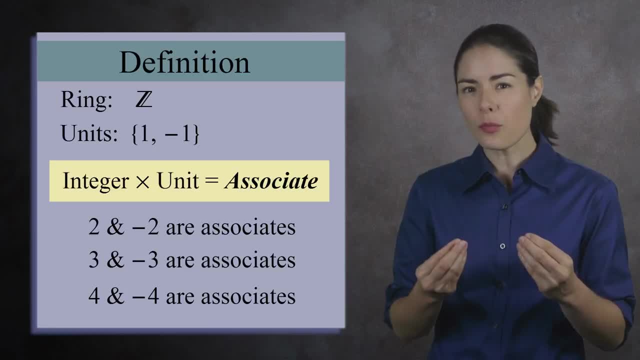 The ideas of units and associates are needed for a more precise discussion of factoring numbers. 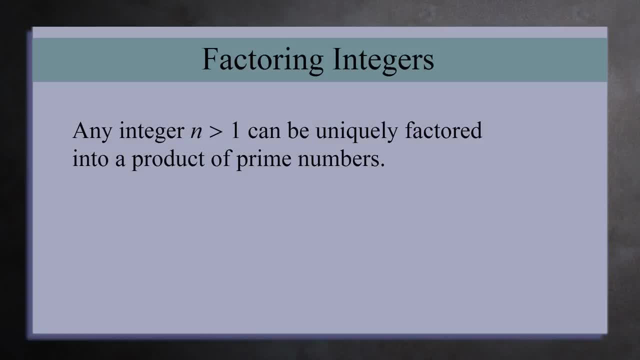 Most people know you can factor any integer greater than 1 uniquely into a product of primes. This is known as a fundamental theorem of arithmetic. We don't include 1 because it's a unit, and units aren't prime, and do not have a unique factorization. For example, we can factor the integer 1 as 1 times 1, 1 times 1 times 1, and so on. But what about the negative integers? Do they have a unique factorization? They do. 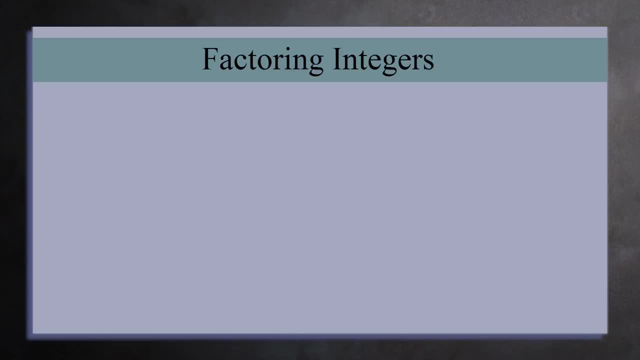 But you need to use units and associates to describe it. For example, negative 12 can be written as 2 times 2 times negative 3. It can also be written as negative 2 times negative 3 times negative 2, or as 2 times negative 2 times 3. We can even factor it as negative 1 times 1 times 2 times 2 times 3. But these factorizations are all related, because 2 and negative 2 are associates, and 3 and negative 3 are also associates. 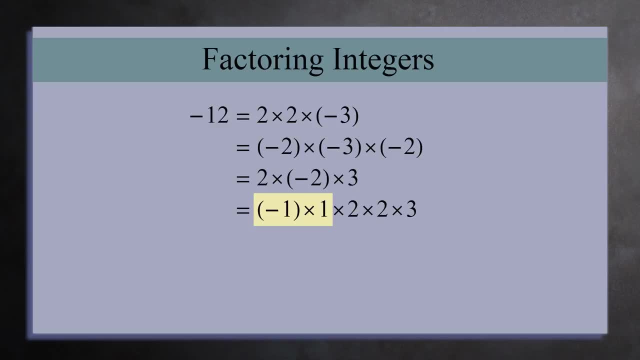 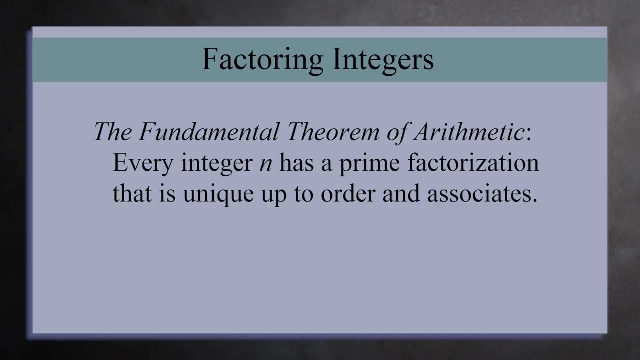 The last factorization just includes a few units thrown in. You can absorb these units into the first factor. If we reorder the factorizations so the associates line up with one another, we see the factorizations are all the same, the only difference being the terms are associates of one another. We often say the factorizations are unique up to order and associates. This is the fundamental theorem of arithmetic generalized to all integers. It applies to every integer except 0 and the two units 1 and negative 1. The problem of finding the units in a ring is a major topic in number theory. 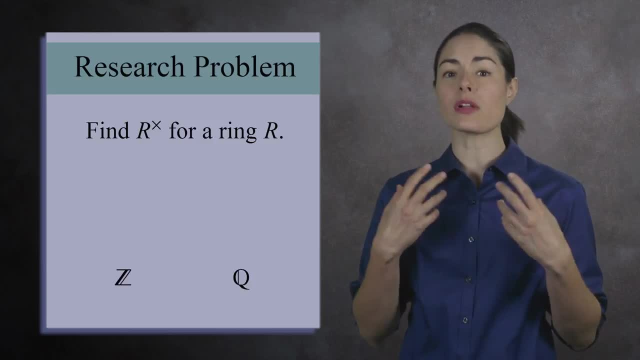 This is because the integers and the rational numbers have been generalized into extensions, called the ring of integers and number fields. 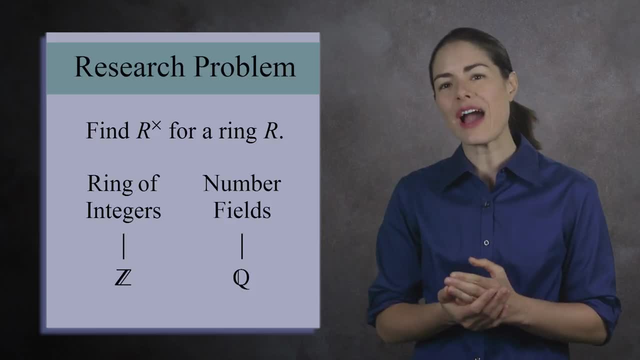 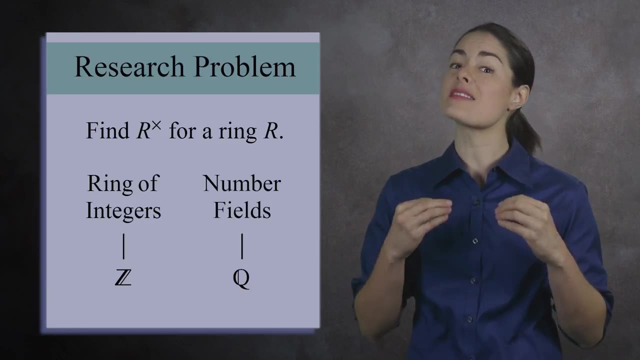 And many problems in number theory require an understanding of how many units there are and what is the structure of this group. Describing the group of units is a difficult problem that is still being researched today. 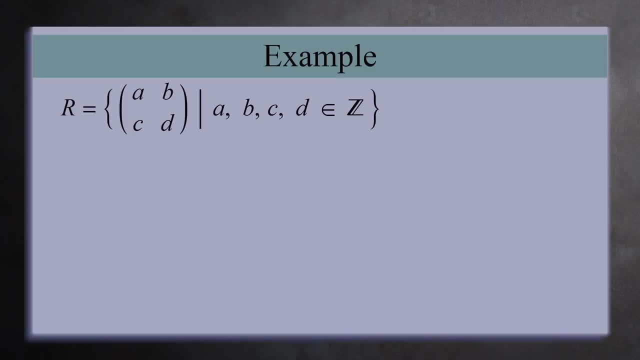 As a final example, look at the ring of 2x2 matrices with integer entries. Most of these matrices do not have an inverse under multiplication. 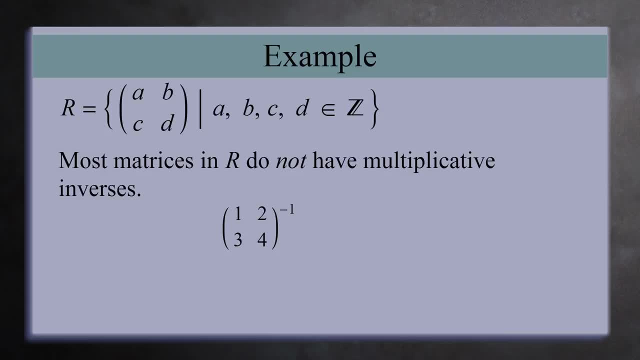 For example, the inverse of the matrix 1, 2, 3, 4 is the matrix negative 2, 1, 3 halves, and negative 1 half. 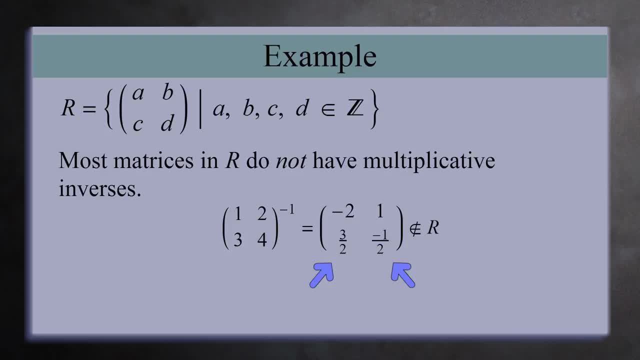 This matrix is not in the ring because two of the entries are fractions. 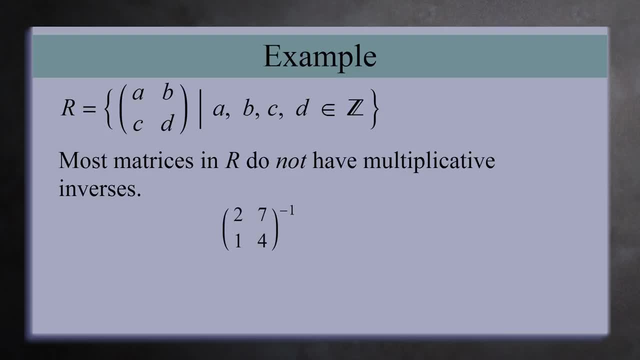 But look at the matrix 2, 7, 1, 4. The inverse of this matrix is 4, negative 7, negative 1, 2, which IS in the ring. 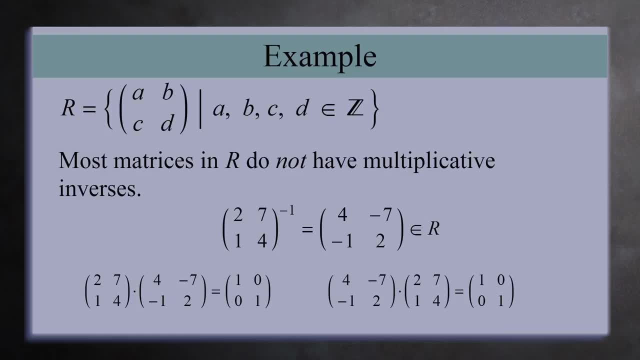 Their product is the identity matrix, regardless of the order, so this matrix is a unit. In fact, this ring has an infinite group of units, the set of all matrices with determinant 1 or negative 1.